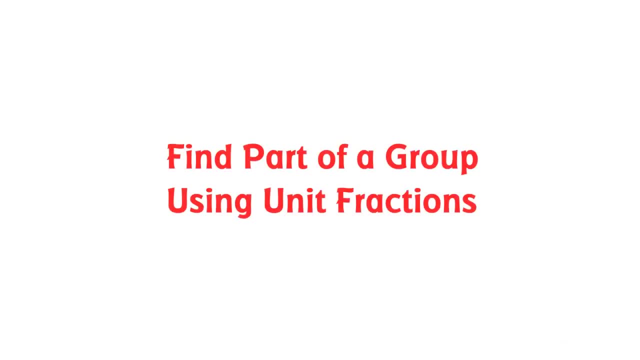 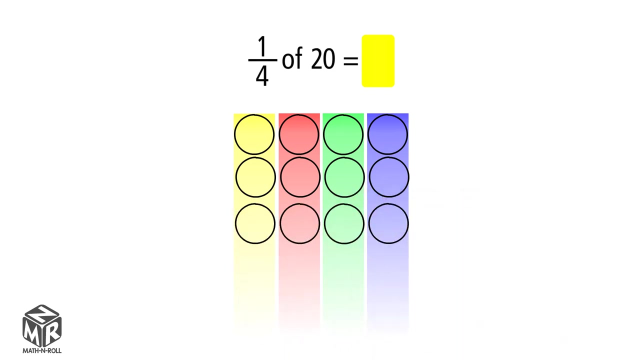 Find part of a group using unit fractions. Since we want to find 1 fourth of the group, we need to have 4 equal groups. Then we draw a row of 4 counters. Continue to draw as many rows of 4 counters until you have 20 counters. Each group represents 1 fourth of 20.. There, 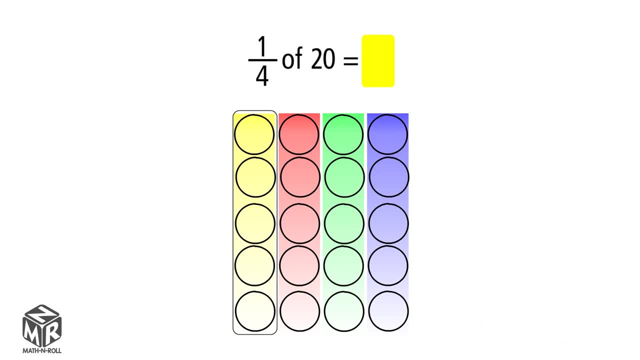 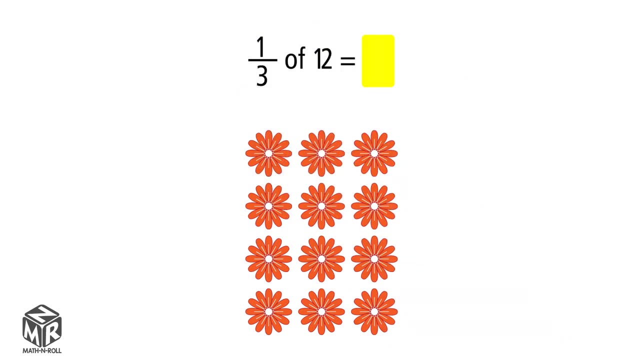 are 5 counters in one group, so 1 fourth of 20 equals 5.. Let's try another example. Use the model to find 1 third of 12.. We need to find 1 third of 12, so we should have 3 equal groups. Let's circle equal groups. 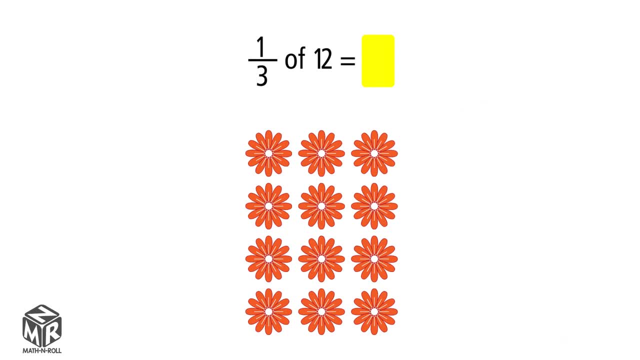 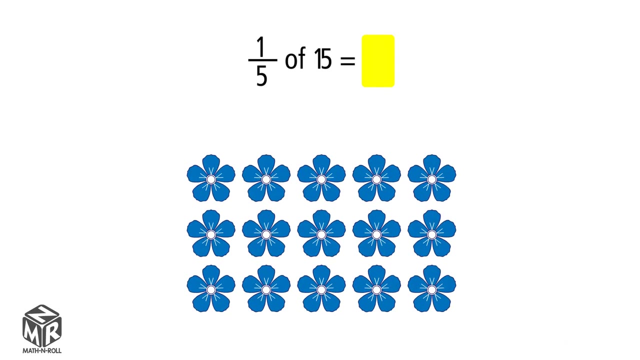 and count the number of flowers in one group. There are 4 flowers in one group, so 1 third of 12 equals 4.. Let's try another example. We need to find 1 fifth of 15, so we need 5 equal groups. Circle equal groups and count the number of flowers in one group. Let's 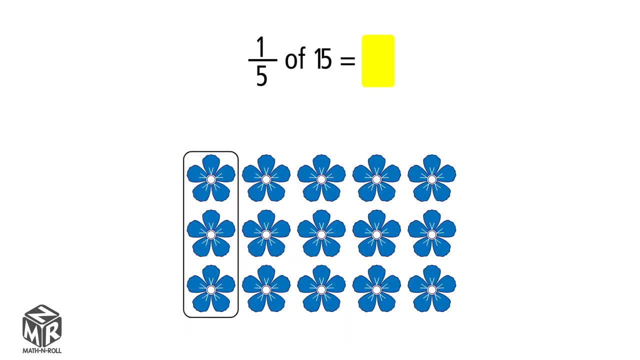 draw a row of 4 counters using unit fractions, Since we want to find 1 fourth of 15, so And 3 equals 3.. Then we add divisible numbers. Şimdi we see that it's not 0 and there is 3 flowers in one group. There are 3 flowers in one group, so 1 fifth of 15 equals 3.. Let's. 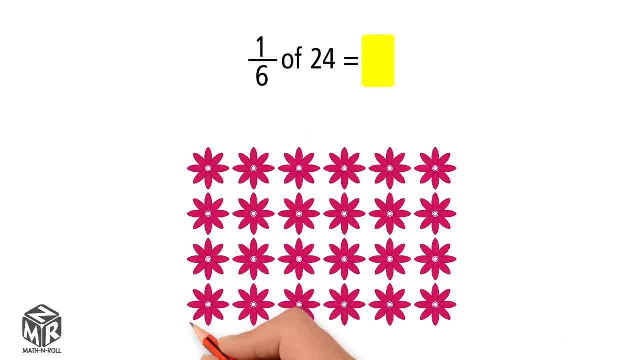 try another example. Use the model to find 1 sixth of 24,. so we need to have 6 equal groups, Circle equal groups and count the number of flowers in one group. There are 4 flowers in one group, so 1 sixth of 24 equals 3.. Let's count the number of flowers in one. 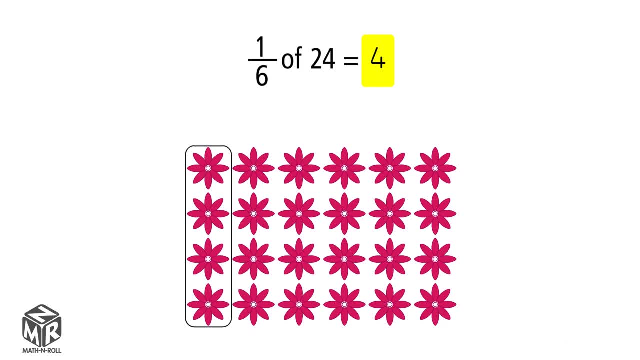 24 equals 4.. If you thought this video was helpful, please leave a like. For more videos like this, please subscribe.